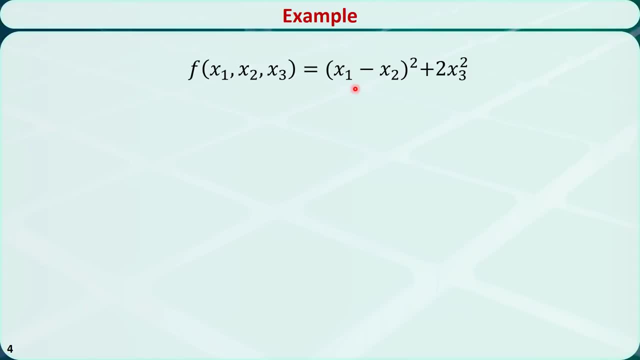 Let's calculate the Hessian matrix of this example: x1 minus x2 squared plus 2 times x3 squared. It has three variables: x1, x2, and x3.. Let's first calculate the first-order partial derivative with respect to x1.. 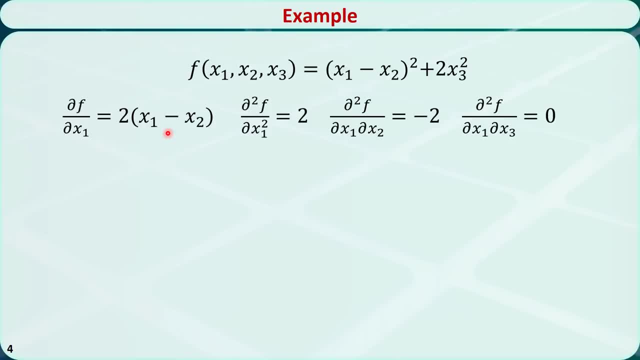 It's 2 times x1 minus x2.. Then we calculate the second-order partial derivative with respect to x1 and x1.. The second-order partial derivative with respect to x1 and x2.. And the second-order partial derivative with respect to x1 and x3.. 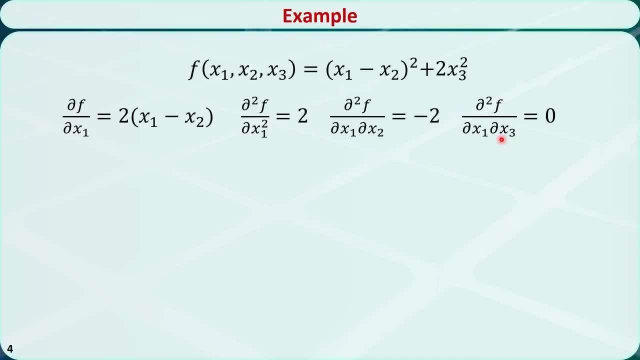 They are 2, minus 2, and 0, respectively. This is the first row of the Hessian matrix. Similarly, we can calculate the second and third row of the Hessian matrix. Finally, this is the Hessian matrix of this function. 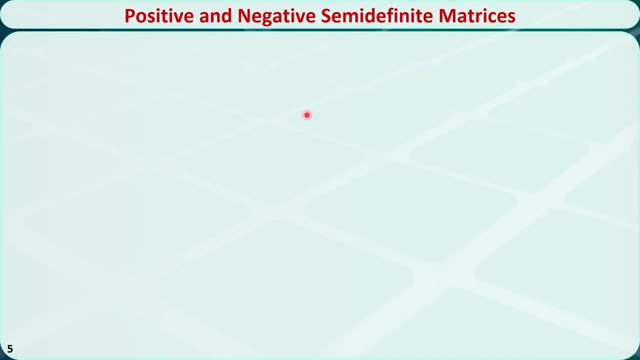 Now let's check the concepts like positive, semi-definite And negative semi-definite matrices. The n by n Hessian matrix H is positive, semi-definite if the scalar resulted from this matrix. multiplication z, transpose times h, times z is non-negative for all nonzero. column. vector z of n real. 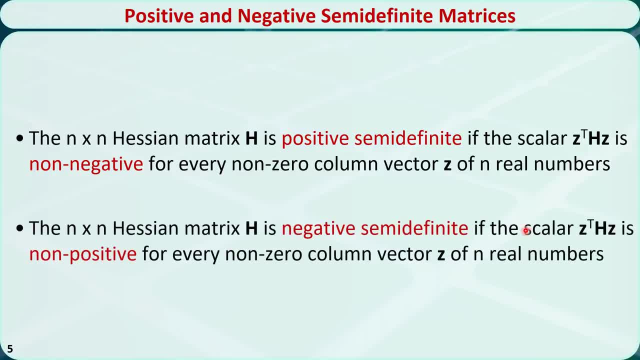 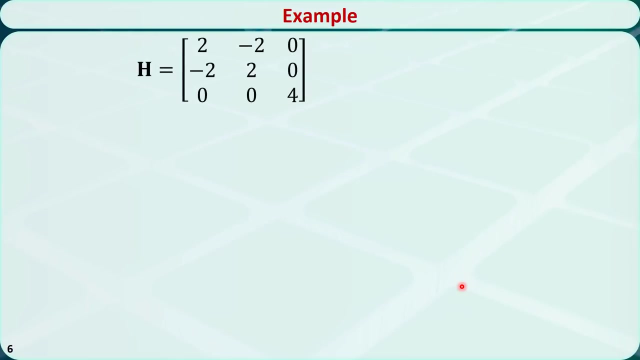 numbers. The n by n Hessian matrix H is negative, semi-definite. if the scalar resulted from this matrix, multiplication is non-positive. Every nonzero column vector z of n real numbers. This explanation still seems complex and difficult to understand. Let's try to see an example. 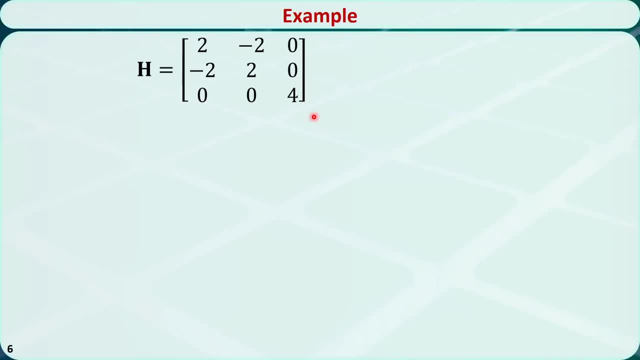 This is the Hessian we got from the previous example. We will determine whether it is positive semi-definite or negative semi-definite. Now let's define a nonzero column, vector, z. It contains 3 numbers: z1, z2, and z3.. 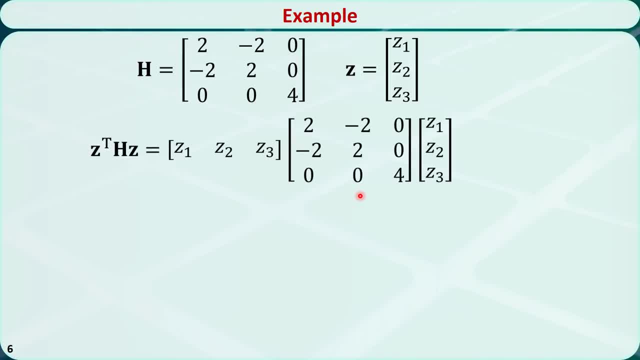 For the matrix multiplication. we can expand it in this form. Then we calculate the product of the first two matrices. This is the 1 by 3 matrix and this is the 3 by 3 matrix. So the result will be a 1 by 3 matrix. 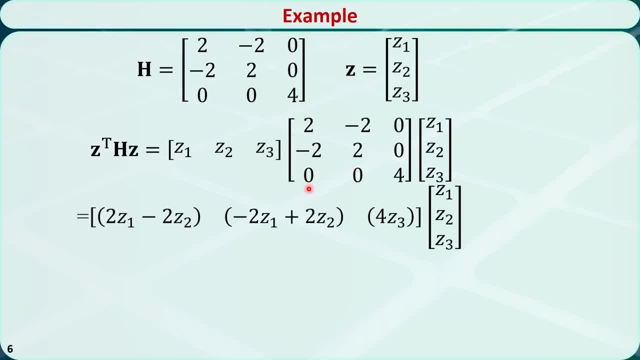 The first element will be the sum of this row times the first column. It is 2z1 minus 2z2.. The second element will be the sum of this row times the second column. It is minus 2z1 plus 2z2.. 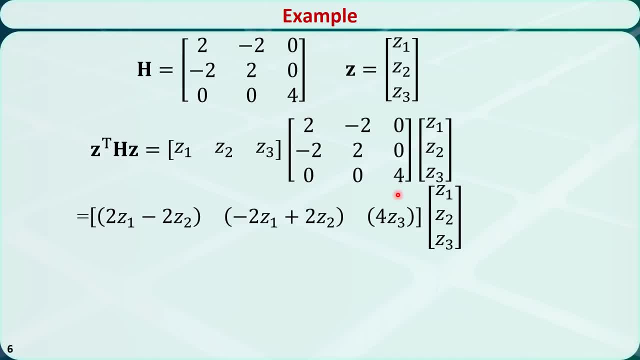 The third element will be the sum of this row times the third column. It is 4z3.. Now let's multiply this row by this column. This is the result. We find that this item must be greater than or equal to 0.. 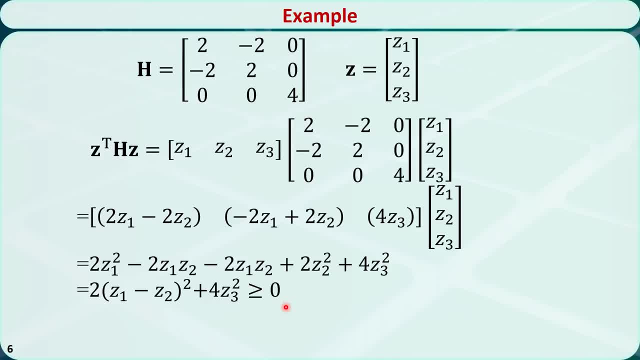 So must this item. Therefore, the sum should also be greater than or equal to 0.. And this hash matrix is positive semi-definite. based on the definition, Finally, we can conclude that this function is a convex function. The method I just introduced can be used to determine whether a function is convex or 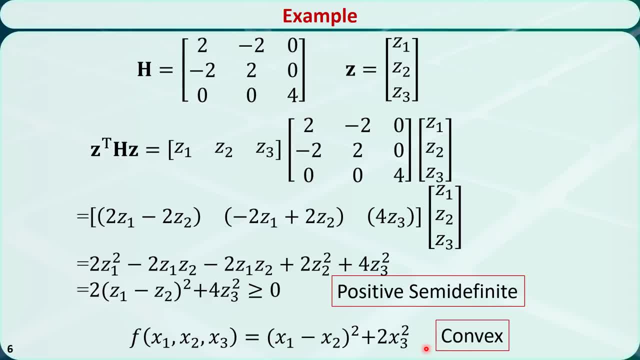 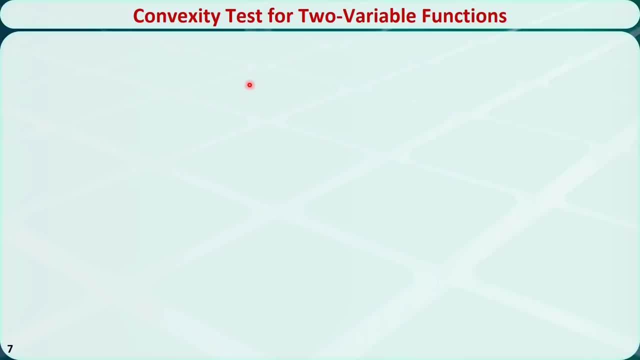 concave. It is applicable to functions with any number of variables. For a function with only two variables, there is an easier way to tell whether it is convex or concave. We need to calculate the second-order partial derivative with respect to x1, only a second-order. 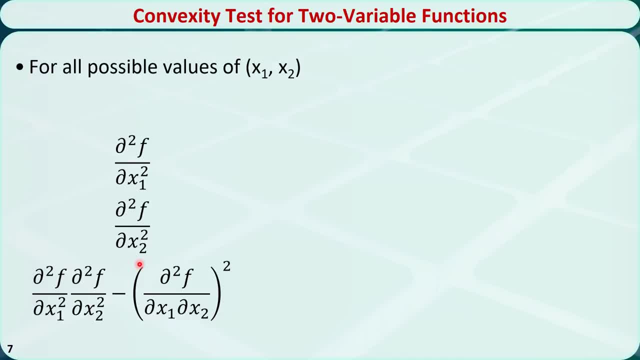 partial derivative with respect to x2 only and their product, minus the second-order partial derivative with respect to x1 and x2 squared. If they are all greater than or equal to 0, for all possible values, of course, we can calculate the two values of x1 and x2.. 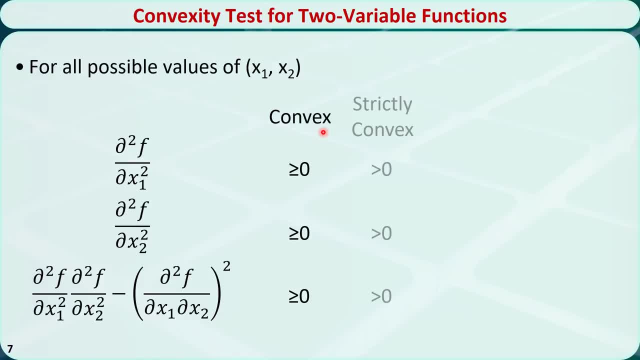 Then the two-variable function is convex. If they are all greater than 0, but not equal to, then the function is strictly convex If the first two are less than or equal to 0, and the last one is greater than or equal. 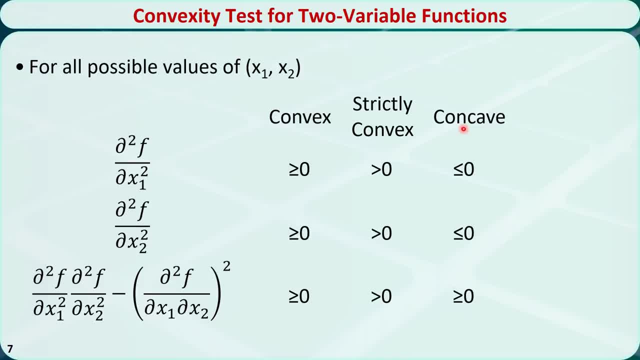 to 0,, then the function is concave. If the first two are less than 0, and the last one is greater than 0,, then the function is strictly concave. With this table in mind, I hope you have learned something.